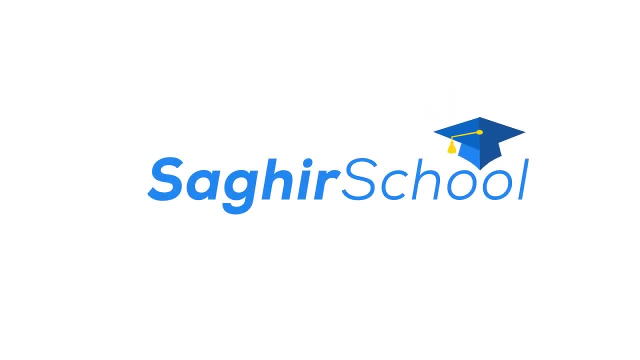 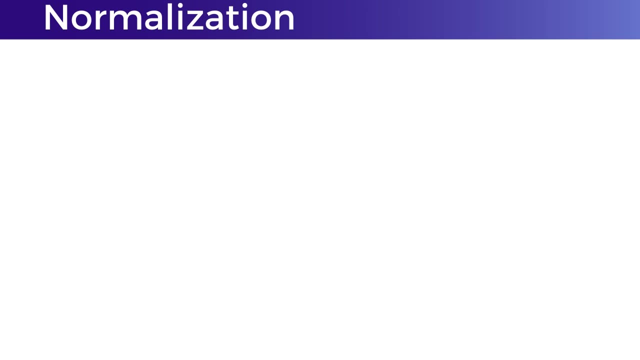 Whenever designing database, the most important thing that you need to do is to take care of the normalization rules. By definition, normalization says it reduces the data redundancy and creates more tables than before. Well, database can handle more tables rather than the tables that are not in normalized form, So making more tables is much more suitable for database. 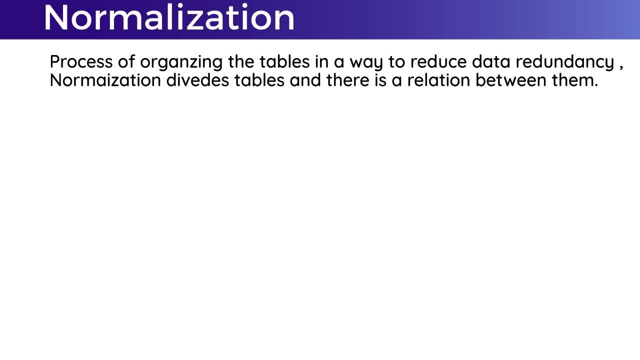 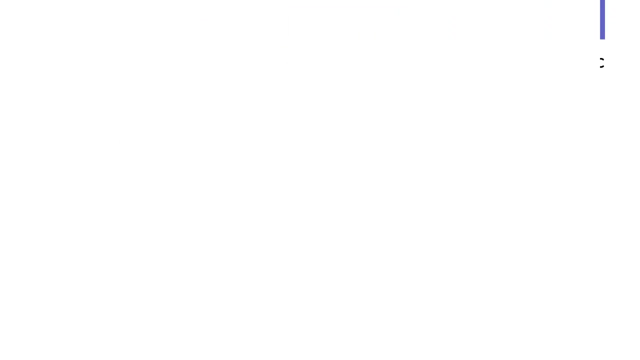 rather than wrong tables. Well, the advantages that normalization brings is flexibility, designs flexibility, database security. Database is much secure with normalization because more tables are formed and there are cases when you need some information to hide from some users, So it counts in data security. reduces data redundancy in a much organized way. These are: 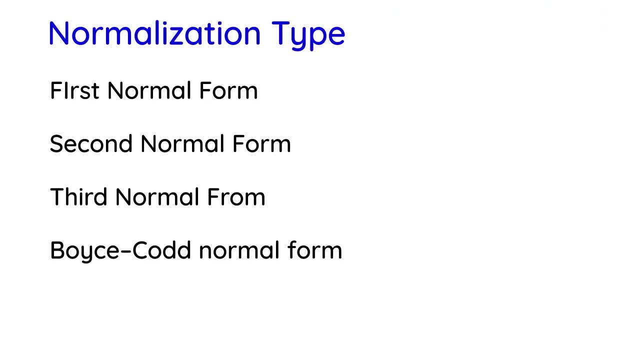 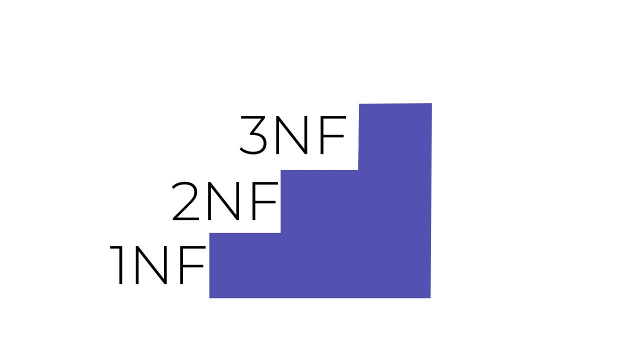 the normalization types we will talk about. By the way, when considering normalization forms, you cannot bypass the previous form, Means first you have to go through first normal form, then second normal form and then eventually third normal form. You cannot bypass the first two and 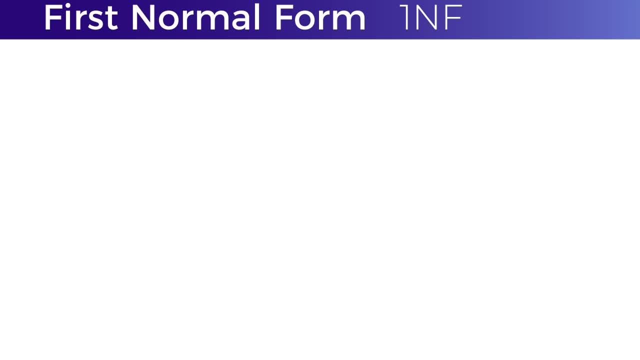 directly go to third one: First normal form. For a table to be in a first normal form it needs two criterias, two things that should not happen in this table. First, no repeating values in a group and no repeating groups in the table. What does that mean, We'll see in the example. 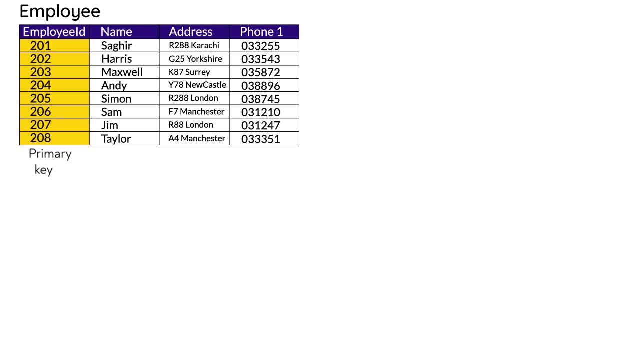 In this example of the employee table. it is in a perfect form, Employee ID is the primary key and it has values of name, address and phone number. So far, so good. What if there's a possibility? when employees having more than one phone number, you can write them like this by: 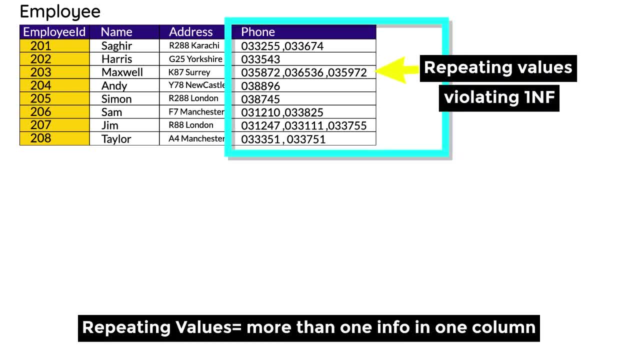 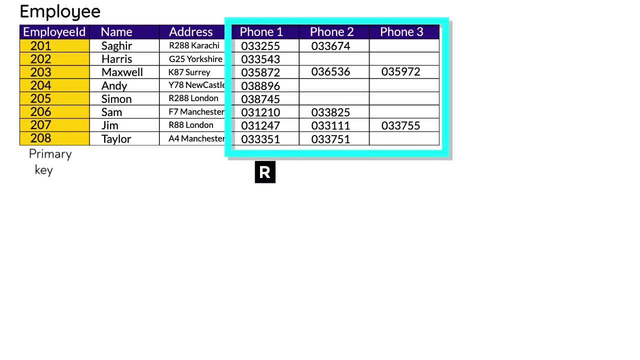 separating with the columns. That's repeating values in a column and it's violating the first normal form. Another possibility of writing it: writing them in different columns, and that's repeating columns. Repeating columns again violates the first normal form. Remember what we gathered from the 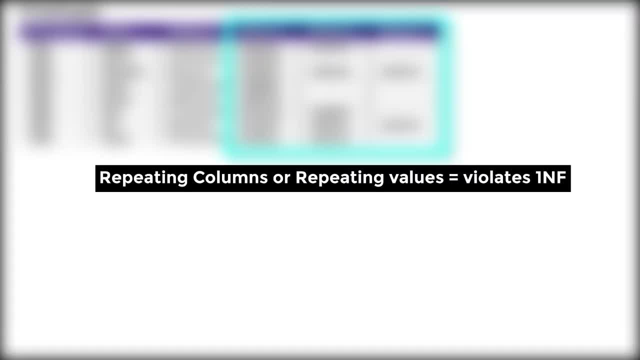 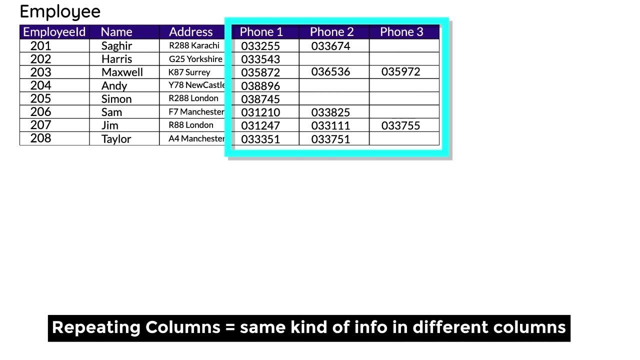 definition of first normal form. Table cannot be in a first normal form if it contains repeating values or repeating columns. Repeating columns are the ones that contain almost same type of information but in different columns. The solution for the problem is that we'll take out the part. 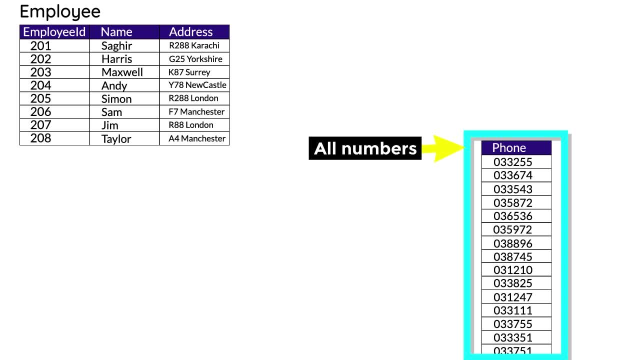 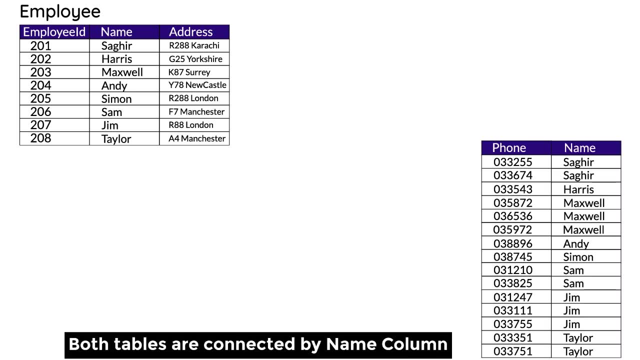 which is creating problem in this table, which are the first normal form. So we'll take out the part which are phone numbers and create a separate table for phone numbers and connect them with the relevant values, which is the name in this case, and then then join both the tables. 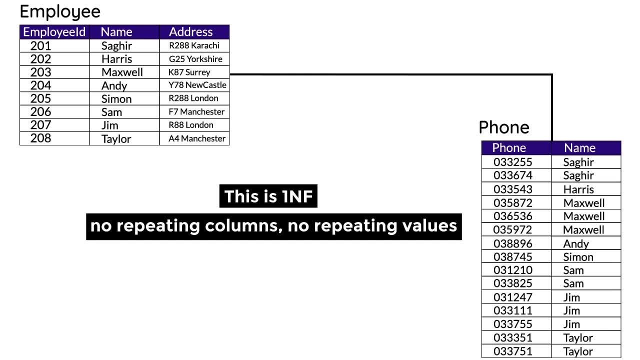 Now it's in first normal form, Although the table have increased from one to two, but there is no repeat values or no repeating columns. Database can easily handle more than one table, but it does not handle repeating values and repeating columns, So we'll need to take care of that. 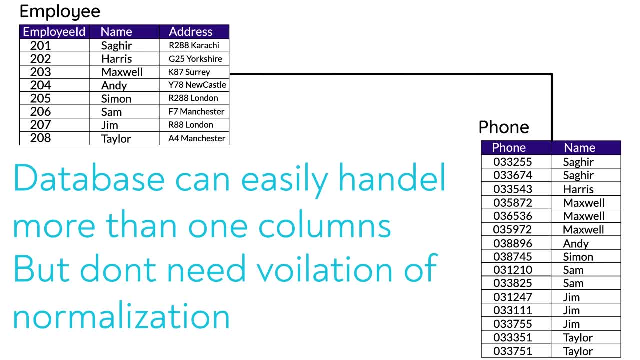 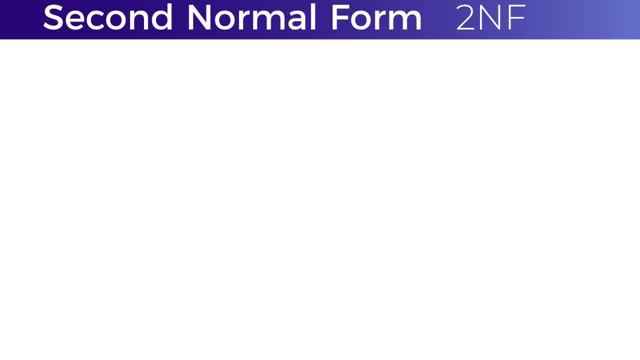 now, if perfectly first normal form condition: the table does not contain in repeating values or repeating columns. for a table to be in a second normal form, it must have three things in it. it should be in first normal form: no partial dependency. partial dependency only can occur when there is a composite key. now what is? 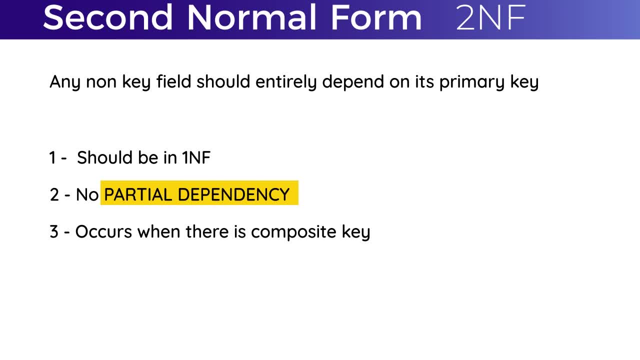 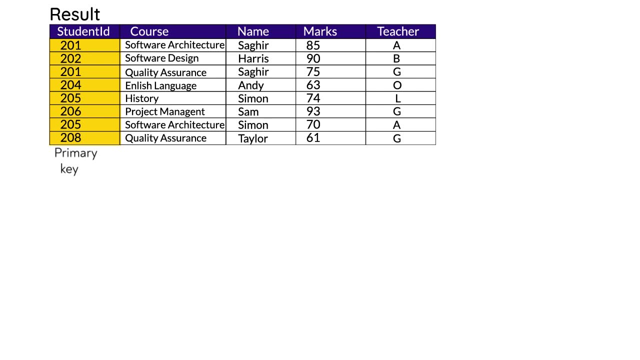 composite key. composite key- composite key is when there is more than one primary key column- means we just cannot identify the result from one particular column. in this example, if we only make a primary key of student ID, we cannot take a record of any student conveniently. because what if we say: give me the? 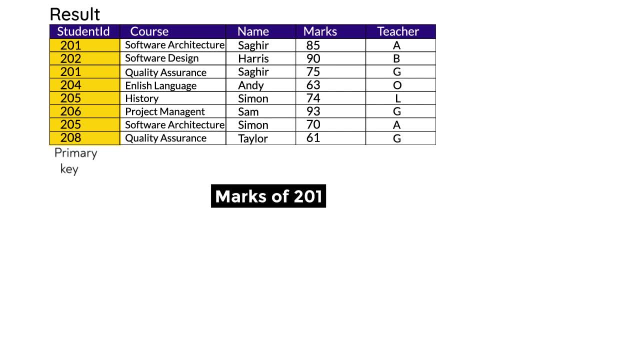 result of 201, now 201. we cannot be sure if we are asking for one 201 software architecture result or quality assurance result. likewise, what if somebody asks us to give a result of 205? 205 is enrolled in history and quality software architecture as well. 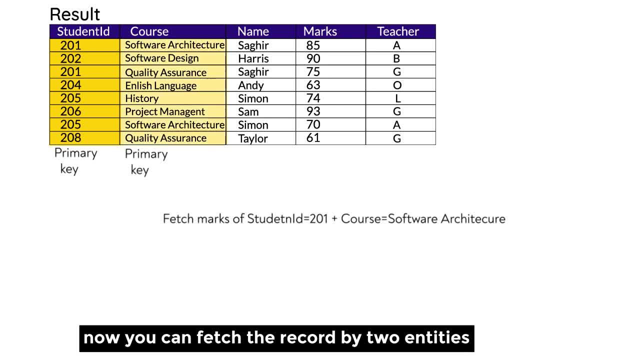 so we make another column as a primary key. now we can easily judge a record. now the question will be: give us a result of a student ID 201 in the course quality assurance or give us a result of a student ID 205 in the course of history? 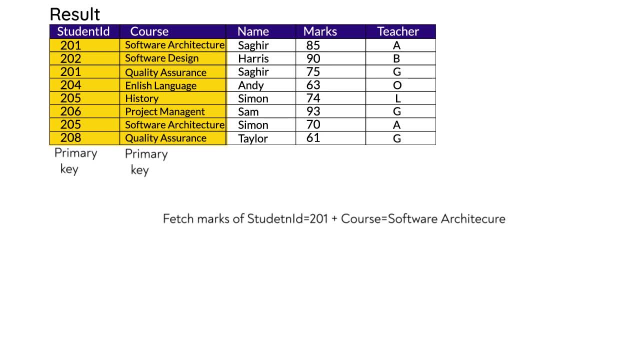 now, student ID was already a primary key. we have also made course as a primary key as well. when there is there are more primary key columns, there are are combinedly called as composite key. now more about partial dependency: student id and course are key columns. name marks and teacher are non-key columns here in this table. now what is partial? 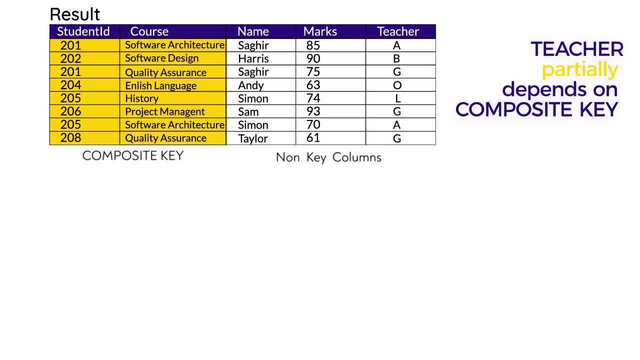 dependency. partial dependency is when any of the non-key column does not depend on all primary key columns, like here. a teacher only depends on the course. what course does the teacher teach? it only depends on course. it does not have anything to do with the student id. both are. 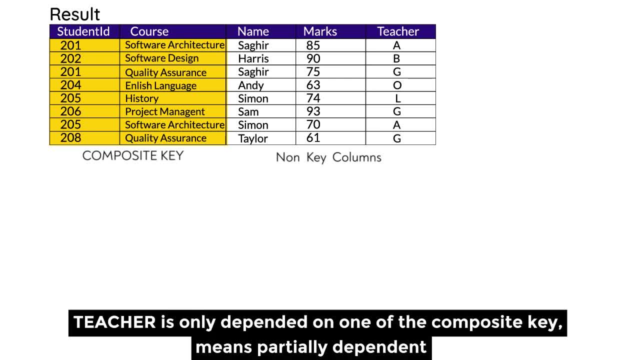 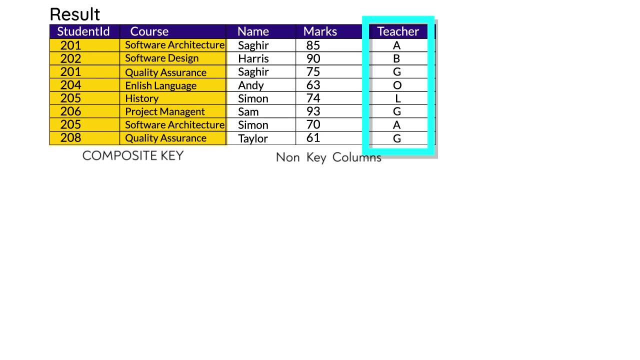 both are key columns. here is a classic situation of the fact that non-key column is only partially dependent on on the key columns. so this is called partial dependency and then when there is a partial dependency, we need to, we need to break that that column into another table which is only partially. 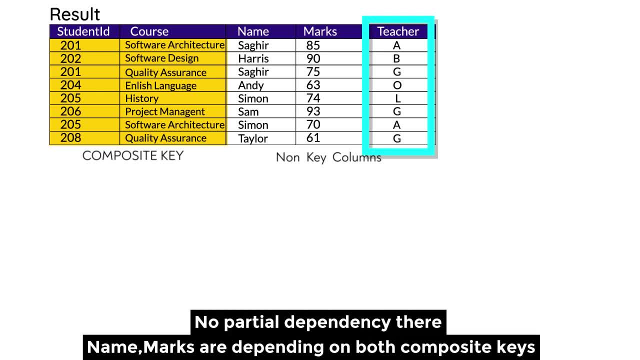 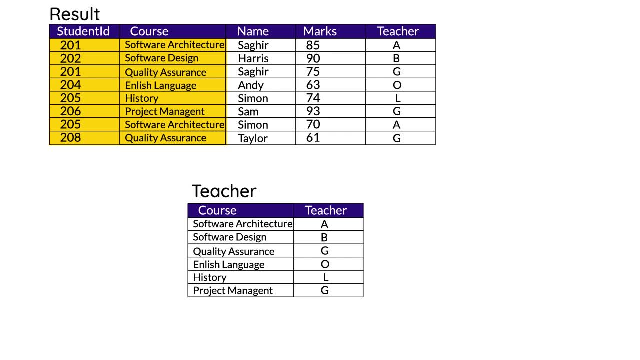 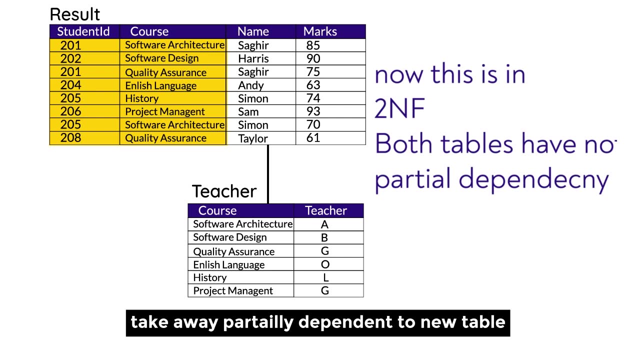 dependent marks and name. both are totally dependent on both the keys. so no need there. you teachers column and taken away from the main table and it is. it is combined with a course column, two tables, and both tables does not have any partial dependency. so it is now considered. 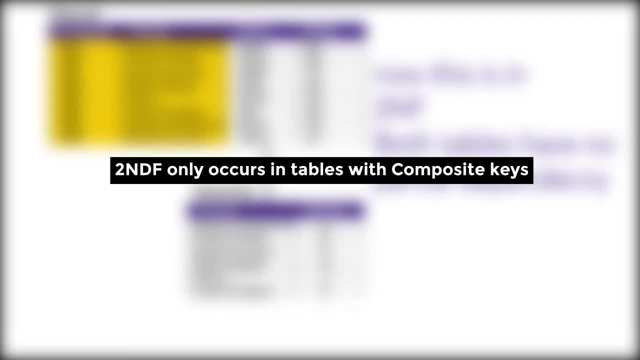 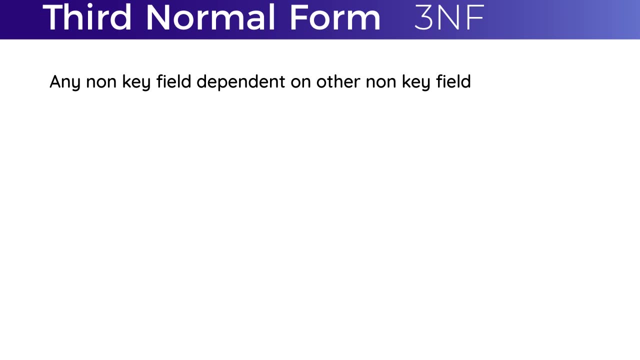 in the second normal form. for a table to be in a third normal form, it must be in a first normal form and second normal form already. third normal form should not have a transit of dependency. what is transitive dependency we will see in the example now. one more thing to note is that if one non-key column can be guessed from other non-key column, 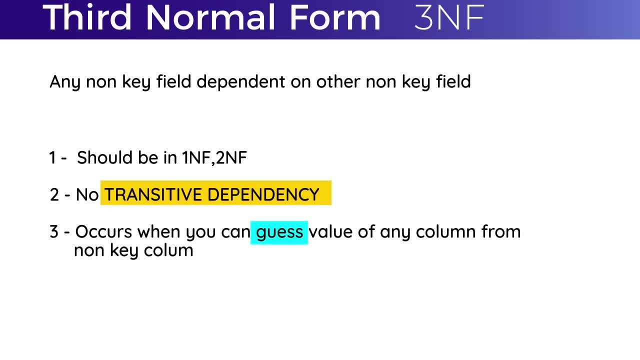 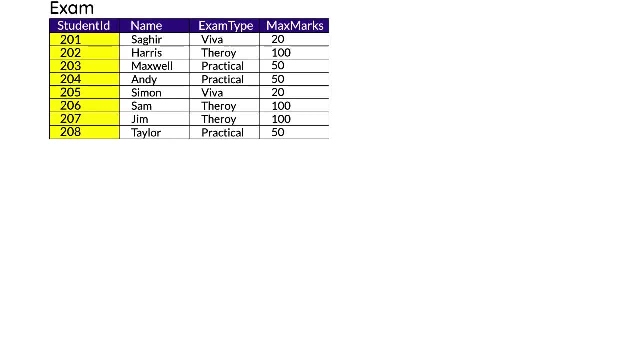 that means it is violating third normal forms rule and we'll need to break the table. we can go through the examples to make it more understandable. in this table, student id is the primary key column and name, exam type and maximum marks are non-key columns. from the table we can guess that if a 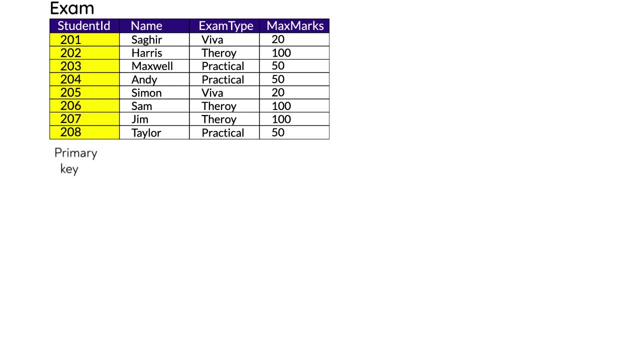 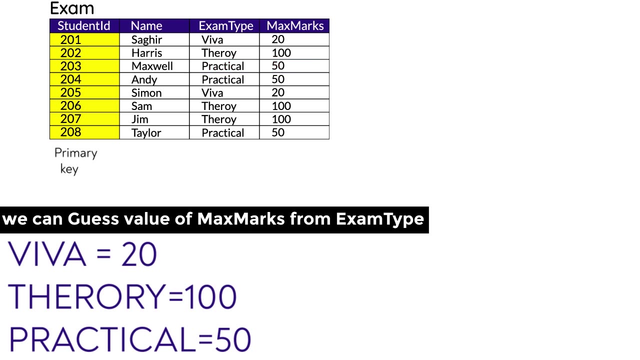 student is opting for viva, means maximum marks will be 20. student is opting for theory, it will be of 100 marks and practical will be of 50 marks. means we can guess the maximum marks column from exam type column. and it also means that maximum marks column is transitively depending on exam. 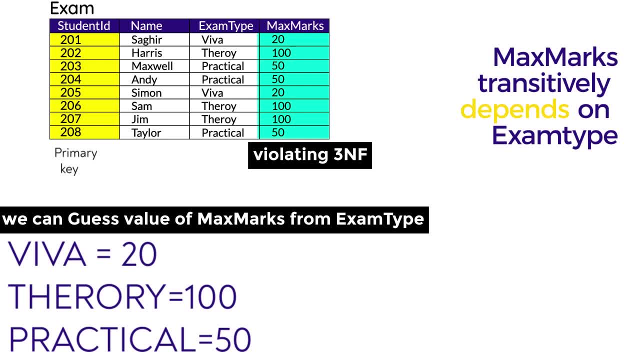 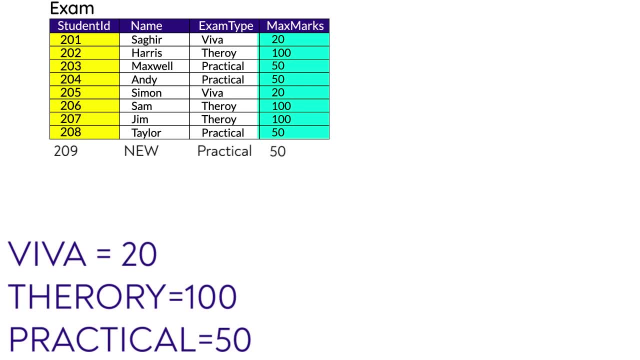 type column. so if some student of id 209 comes and he's opting for practical exam, we'll already know the maximum marks of practical would be 50. this is the classic case of violating third normal form. we will break the maximum marks column and put it in the another table. now it's not in third.